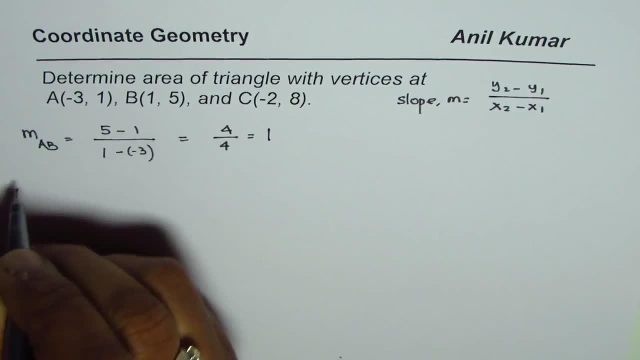 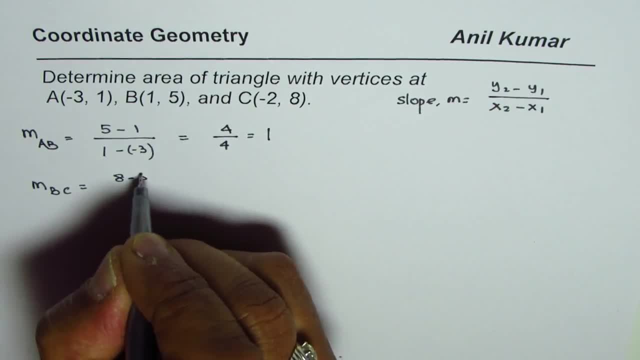 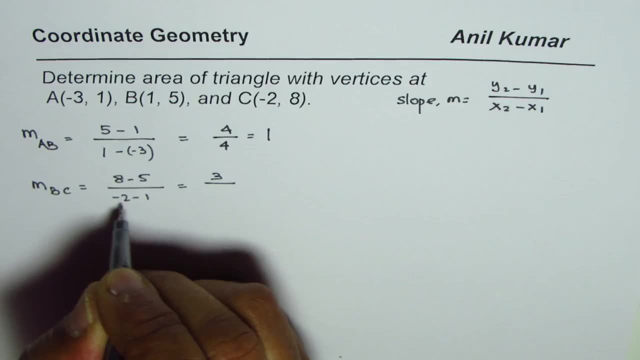 1.. So that is 1 minus 1.. Since slope between c and c is 8 minus 5, divided by minus 2 minus 1, 8 minus 5 is 3 and minus 2 minus 1 is minus 3.. We get slope of minus 1.. Now, since these, 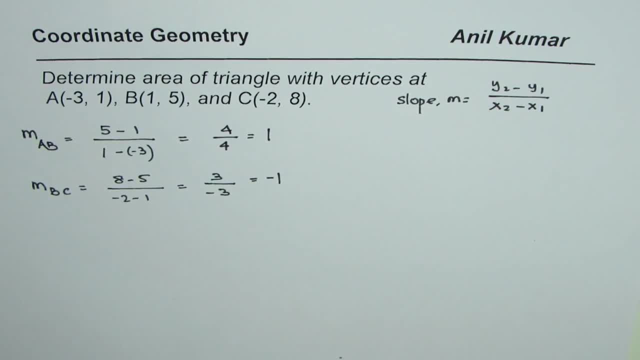 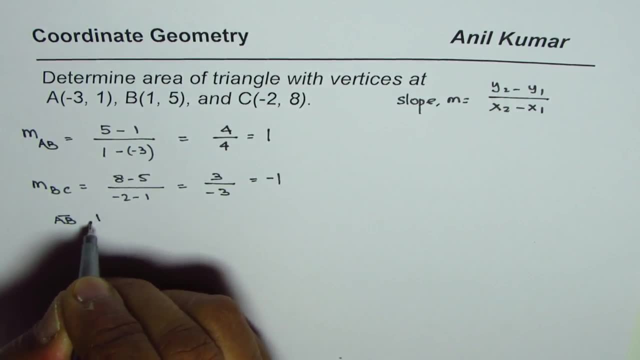 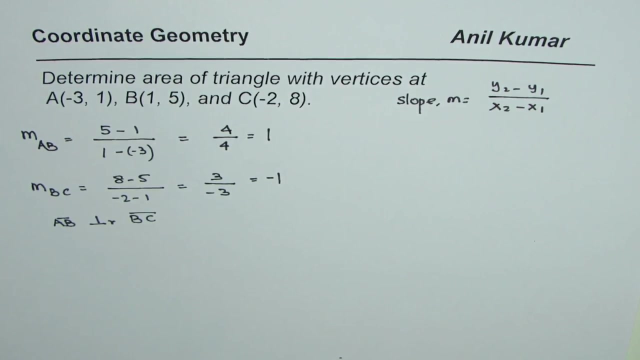 two slopes. when you multiply you get minus 1, they are negative, reciprocal, and therefore we can see that line ab is perpendicular to bc, to b, c. is that okay? so we indeed have a right triangle, okay. so what i'm trying to say here is that if you sketch this triangle, so so these two lines are perpendicular, right. so i'm just. 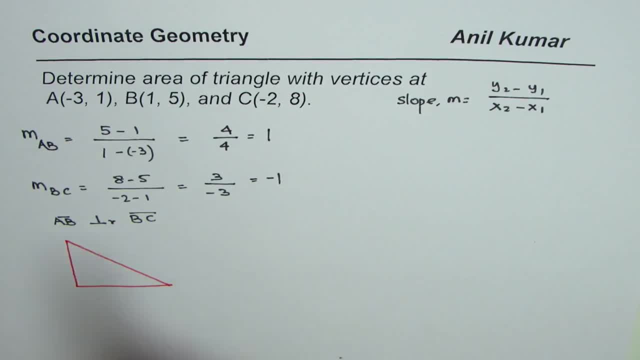 approximately just drawing right. so we are saying a, b and b, c are perpendicular, so b is the common point here and we have these points as a and c, correct? so that is the kind of triangle you have where we have right angles at b, correct? so that clearly shows that area could be written as: 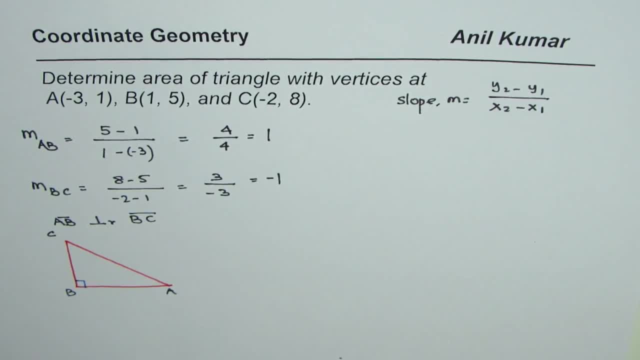 as you know, half base into height, correct? so area is half base into height. we'll do the calculations on this side. so area equals to half of. we can consider a- b as the base right. so we'll take magnitude of a, b times height will be b- c. 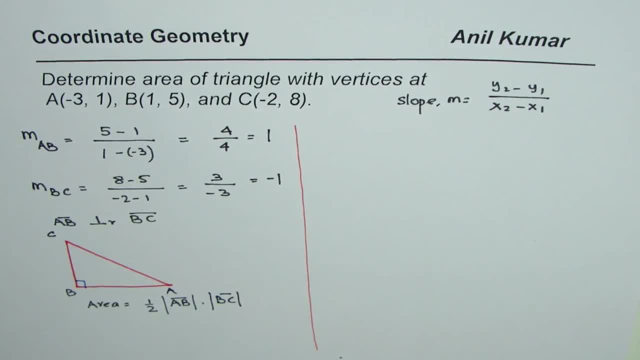 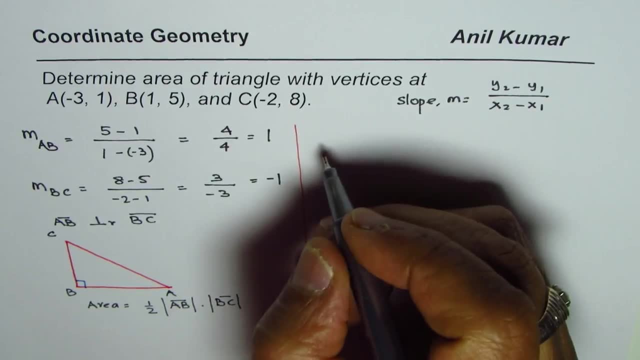 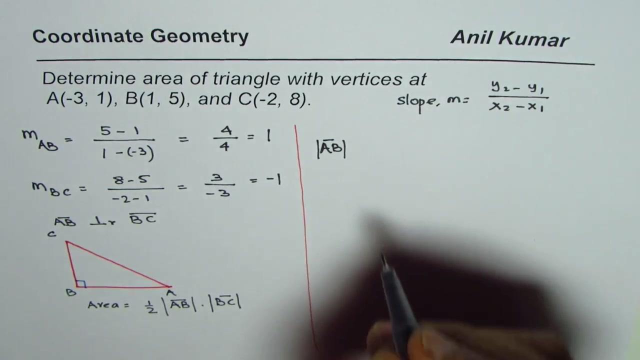 right. so b- c will be the height for us. so that is the area. so to find the area, we need to find length a- b and length b- c. so let's find the length a- b. so what is the length of the side a- b? we'll use the formula which is square root of. let me write down formula first. 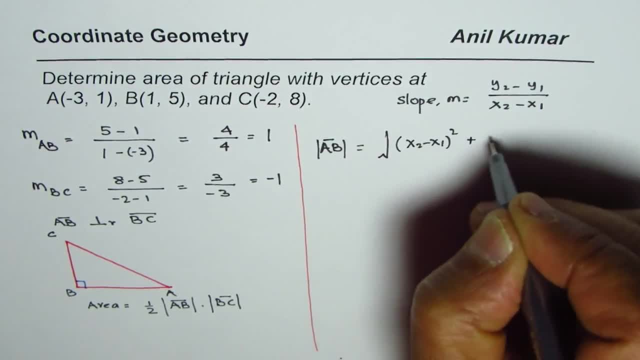 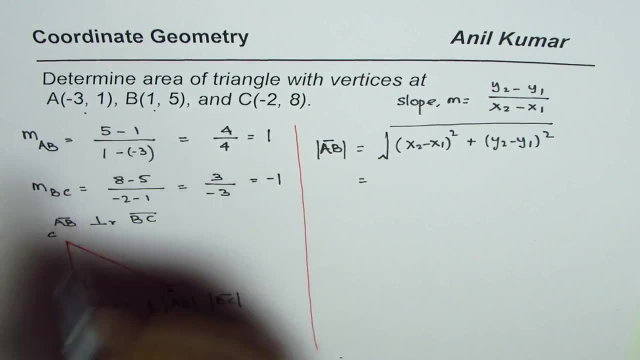 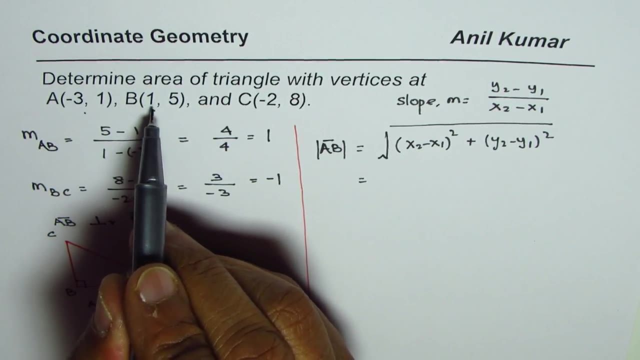 here: x 2 minus x 1 whole square, plus y 2 minus y 1 whole square. correct, that's the formula for a, b, 5, x, x, 1, y 1. let's take a, y, x, 2, y 2 as b. in that case it will be 1 minus square root of.